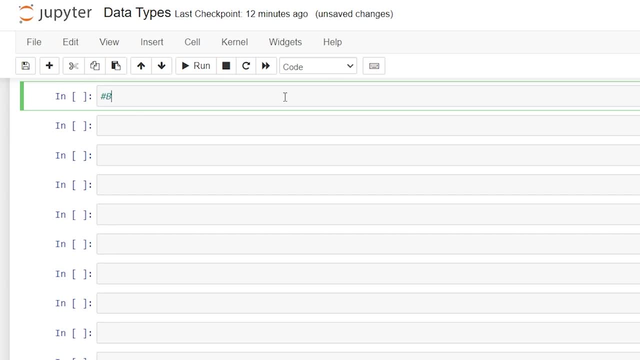 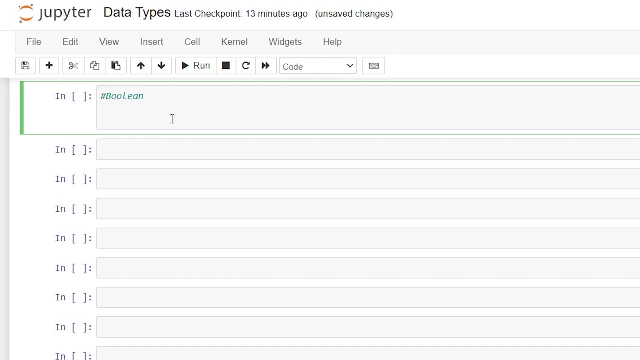 work with it. So let's say boolean values. So we'll say boolean. The boolean data type only has two built-in values: either true or false. So let's go right down here and say type: true, And when we run this it'll say: 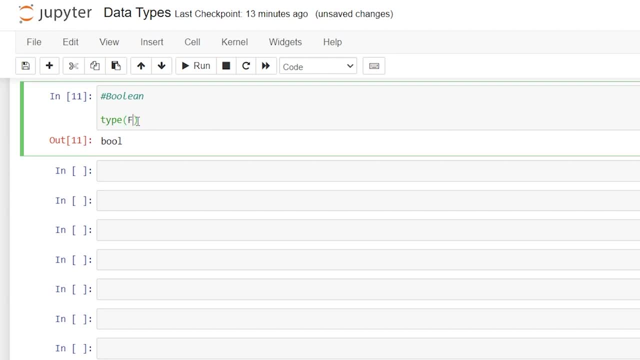 bool, which stands for boolean. We can do the exact same thing with false, and that is also boolean, And this can be used with something like a comparison operator. So let's say one is greater than five And let's check this, This is giving us a boolean, And if we do this, it's going to give us. 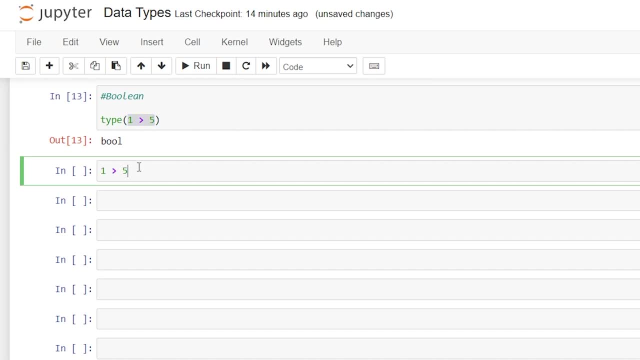 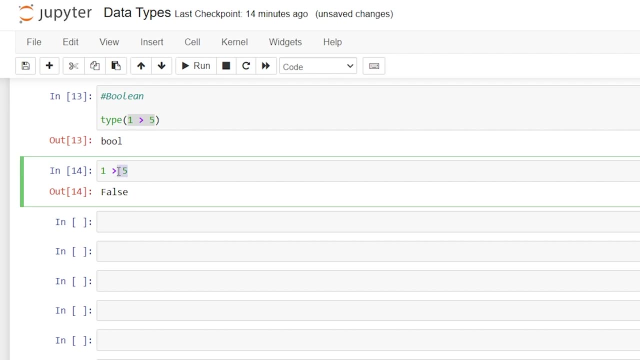 boolean, because it's telling us whether one is greater than five. Let's bring that right down here. This will give us a false. So it's telling us that one is not greater than five. And just as we got a false, we can say: one is equal to one, And this should give us a true. So now let's take a. 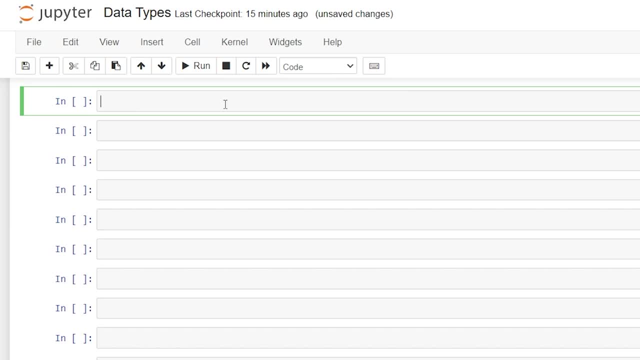 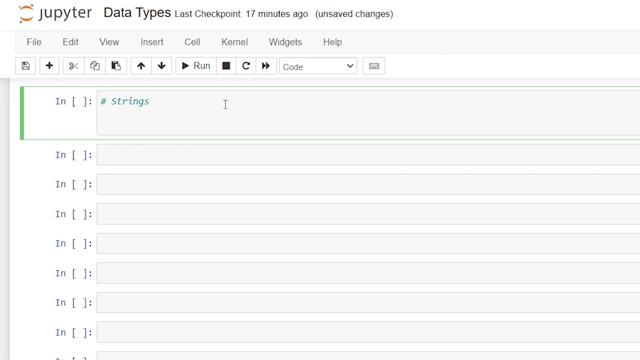 look at our sequence type data types, And that includes strings, lists and tuples. Let's start off by looking at strings. In Python, strings are arrays of bytes representing unicode characters. When you're using strings, you put them either in a single quote, a double quote or a triple quote. I call them apostrophes. It's just what I was. 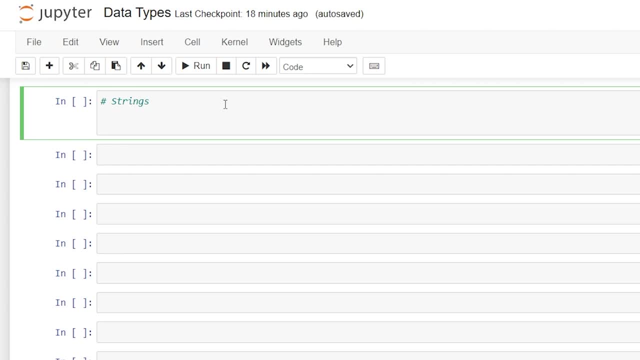 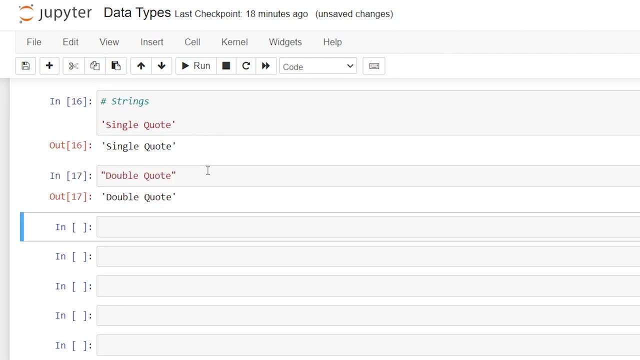 raised to call them, But most people who use Python call them quotes. So right here we have a single quote, And that works well. We can do a double quote, And that works also, And, as you can see, they are the exact same output. And then we have a triple quote, just like this, And this is: 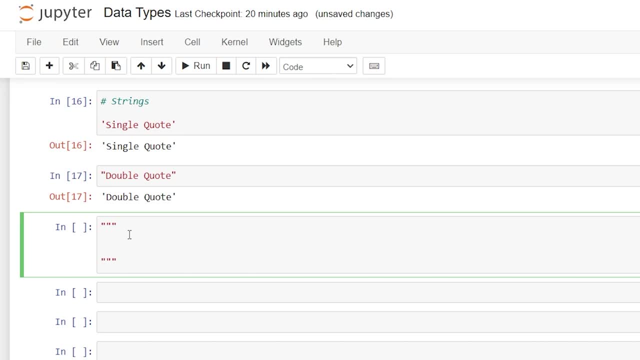 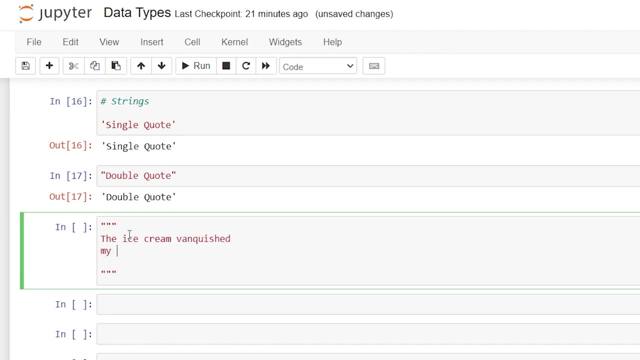 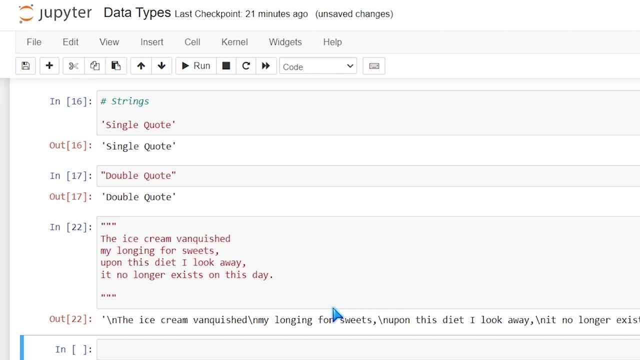 called a multi-line, So we can write on multiple lines here. So let's write a nice little poem. So we'll say: the ice cream vanquished my longing for sweets Upon this diet. I look away. It no longer exists on this day, And then if we run that, it's going to look a little bit weird, It's basically giving. 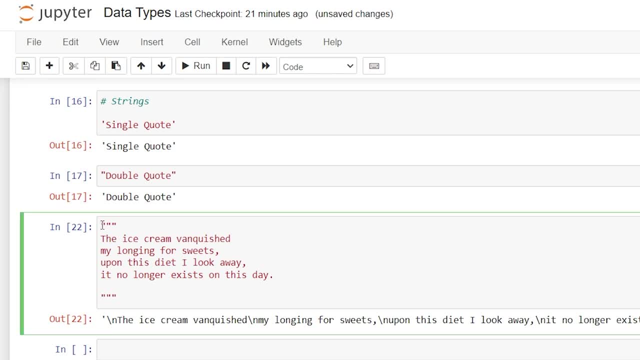 us the raw text, which is completely fine. But let's call this a multi-line And we're going to call this a variable multi-line And we're going to come down here and we're going to call this a variable multi-line And we're going to go down here and say print. And before I run this I have to. 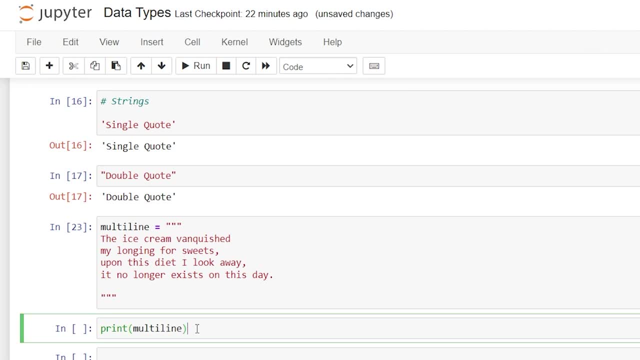 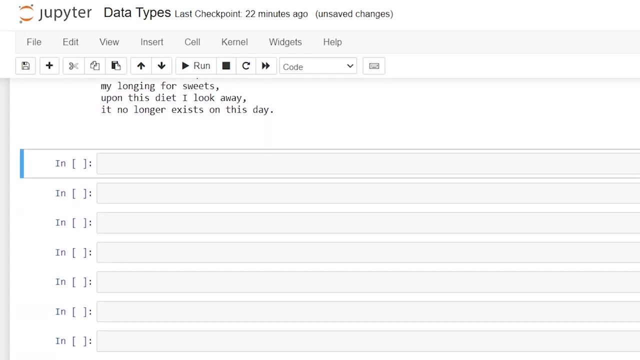 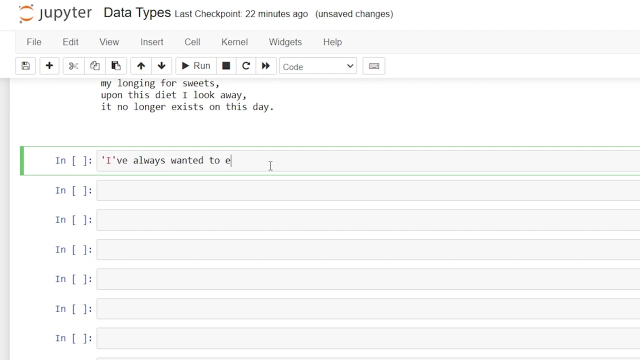 make sure that this is ran. So now let's print out our multi-line, And now we have our nice little poem right down here. Now something to know about these single and double quotes is how they're actually used. So if we use a single quote and we say: I've always wanted to eat a gallon of ice. 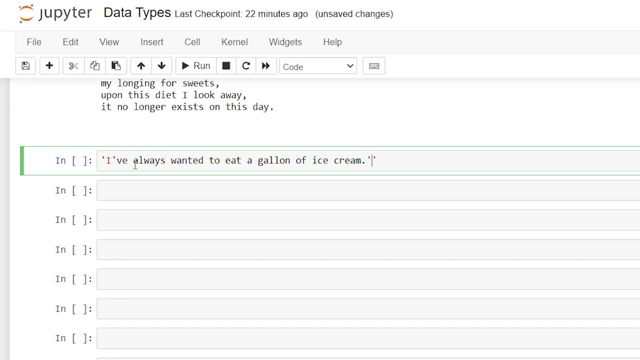 cream And then we do an apostrophe at the end. Obviously, something went wrong here. What went wrong is when you use a single quote and then within your text, within your sentence, you have another apostrophe. It's going to give you an error. So what we want to do is, whenever we have 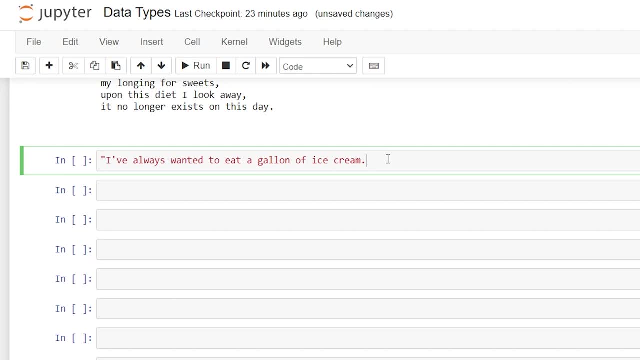 a quote within it, we need to use a double quote. These double quotes will negate any single quotes that you have within your statement. They won't, however, negate another double quote, So you need to make sure you aren't using double quotes within your sentence. If you want to do something like. 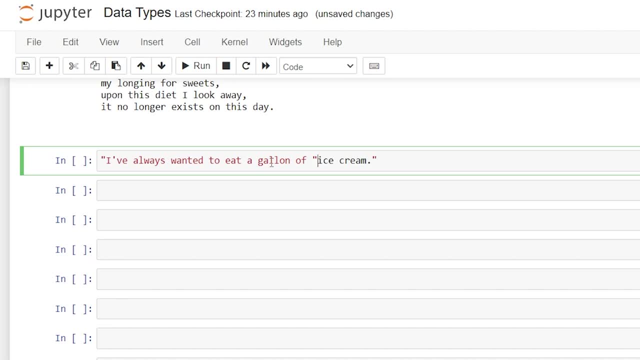 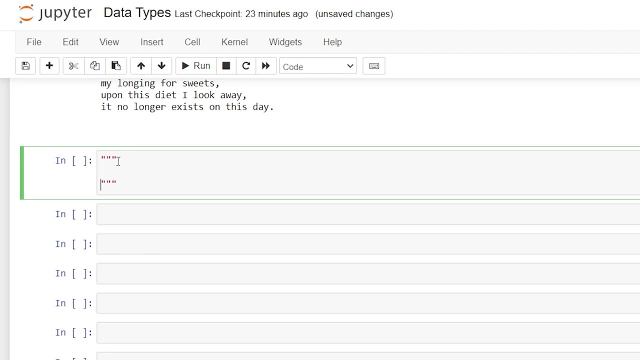 that you need to use the triple quotes like we did above, So we can do double, double and then let's paste this within it And anything you do within these triple quotes will be completely fine. as long as you don't do triple quotes within your triple quotes, We'll say this is wrong. So, even though it's between, 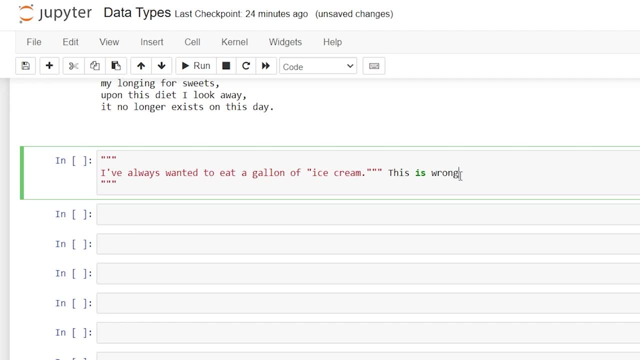 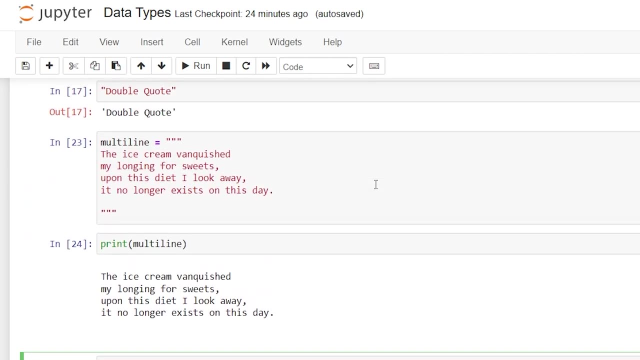 these two triple quotes. it doesn't work exactly. Again, you just have to understand how that works. You have to use the proper apostrophes or quotes within your string And just to check this, we can always say here's a double quote, And then we can do double, double and then let's paste this within. 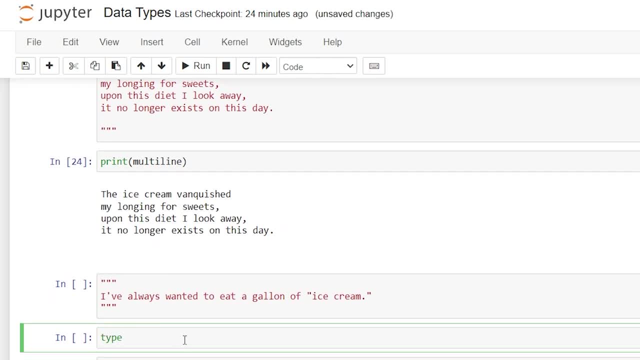 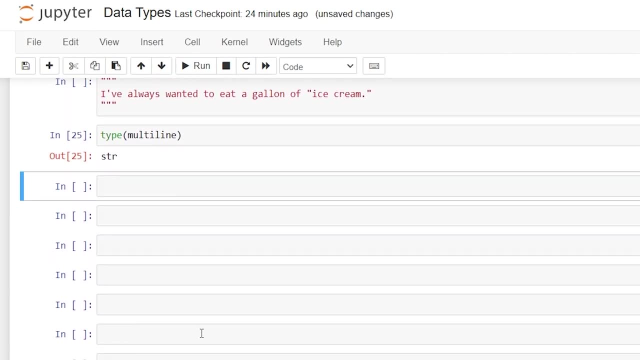 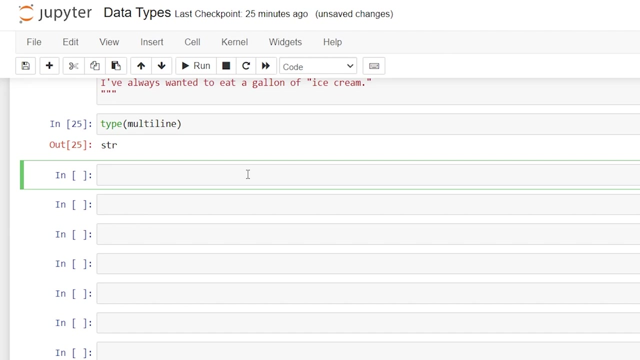 our multi line. We can always say type of multi line, And that is still a string. One really important thing to know about strings is that they can be indexed. Indexing means that you can search within it, and that index starts at zero. So let's go ahead and create a variable And we'll 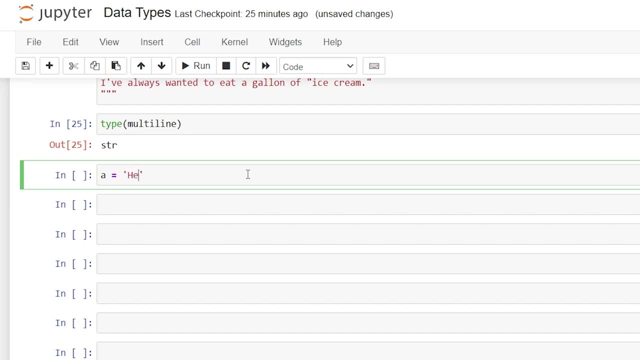 just say: a is equal to: and let's do the all popular hello world. Let's run this. And now, when we print out the string, we're going to say a and we're going to do a bracket, And now we can search throughout our string using the index. So all you have to do is do a colon. I'm going to say five. 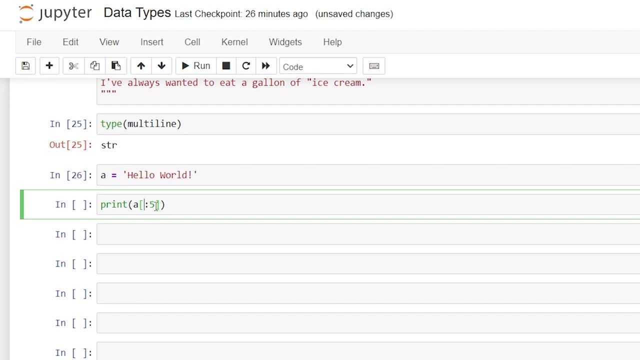 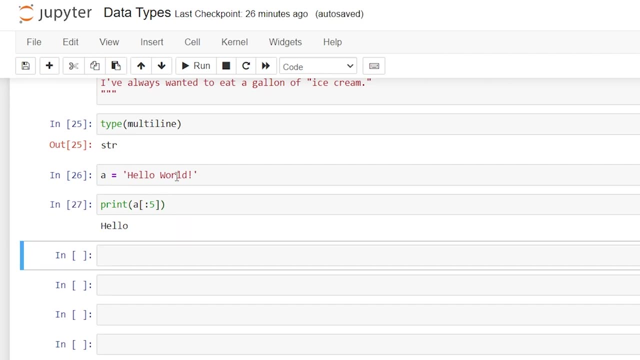 What this is going to do is going to say zero, position zero all the way up to five, which should give us the whole hello. I believe Let's run this and it's giving us the first five positions of this string. We can also get rid of the colon and just say something like five, And then, when we run, 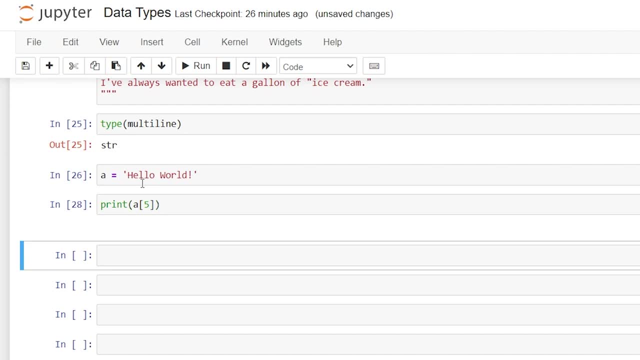 this. it's actually going to give us position five, So we're going to do a colon and we're going to. So this is 0,, 1,, 2,, 3,, 4, and then 5 is the space. Let's do 6 so we can see the. 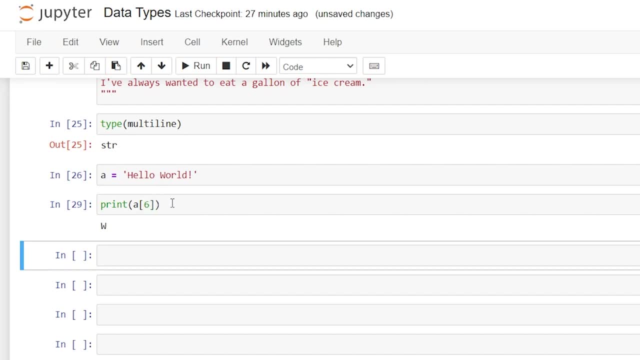 actual letter and that is our W. We can also use a negative when we're indexing through our string. So we could say negative 3 and it'll give us the L because it's negative 1,, 2, and 3.. We can also specify a range if we don't want to. 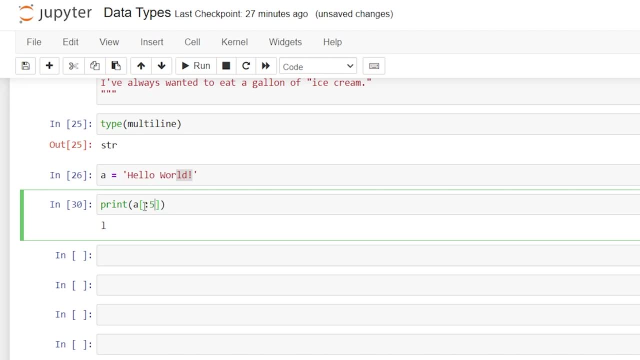 use the default of 0.. So before we did 0 to 5 and it started at 0 because that was our default, but we could also do 2 to 5.. Let's run this, and now we go position 0,, 1, and then we start at 2,, L, L, O. Now we can also multiply strings and 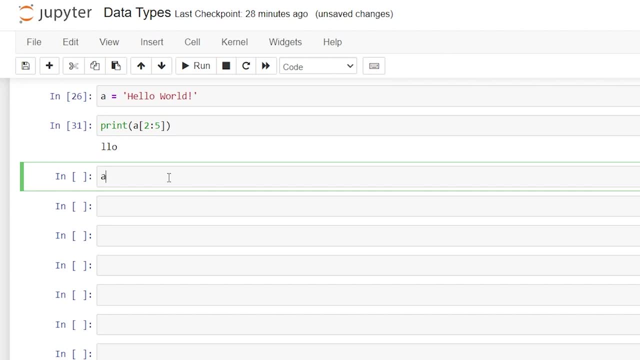 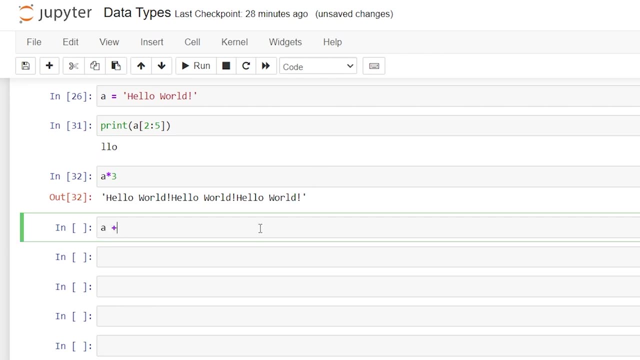 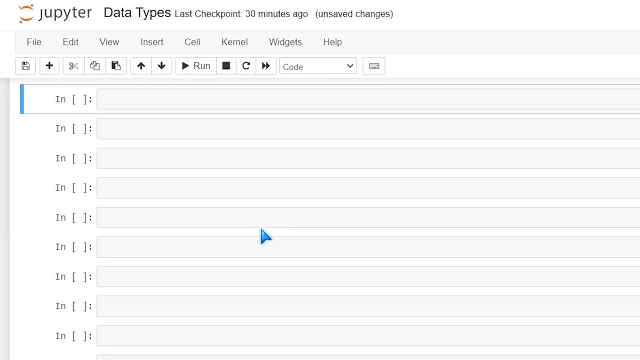 we have this A hello world, So we can do A times 3 and if we run this, it'll give us hello world three times. And we can also do A plus A, and that is hello world, hello world. Now let's go down here and take a look at lists. Lists are: 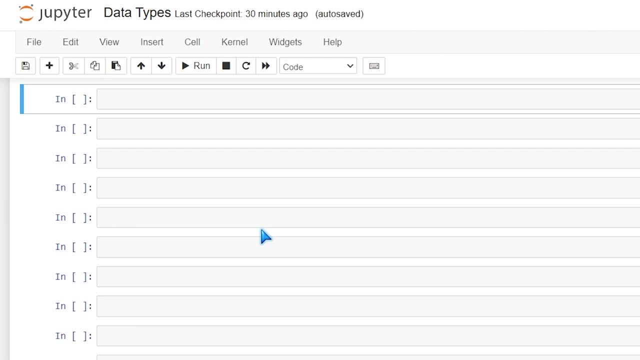 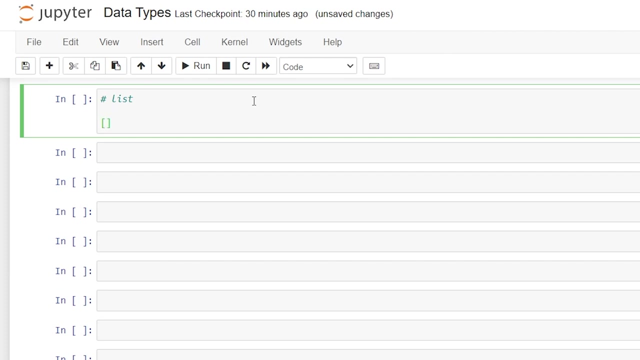 really fantastic because they store multiple values. The string was stored as one value, multiple characters, but a list can store multiple separate values. So let's create our very first list. We'll say list really quickly and then we'll put a bracket, and a bracket means this is going to be a list. There are other. 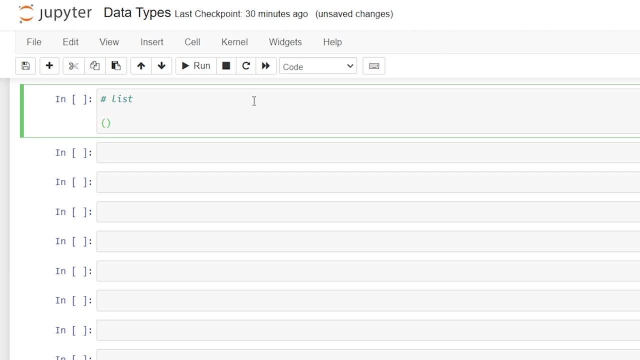 ones like a squiggly bracket and a parentheses. These denote that they are different types of data types. The bracket is what makes a list a list. So, to keep it super simple, we'll say 1,, 2,, 3 and we'll run this, And now we have a. 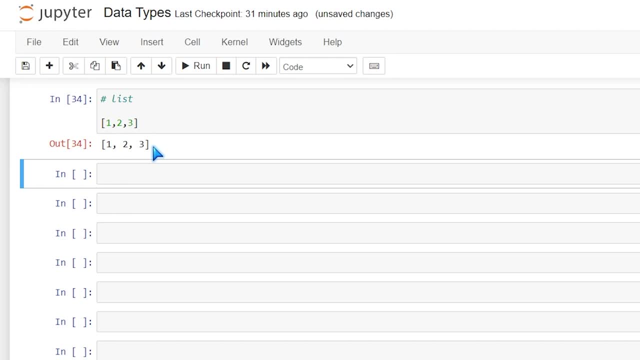 list that has three separate values in it. The comma in our list denotes that they are separate values, and a list is indexed just like a string is indexed. So position 0 is this 1,, position 1 is the 2, and position 2 is the 3.. Now, when we 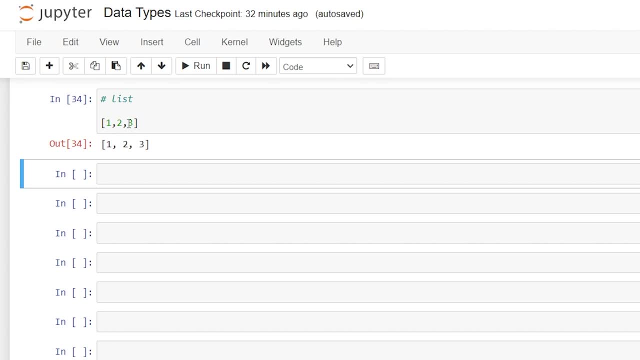 made this list, we didn't have to use any quotes because these are numbers. but if we wanted to create a list and we wanted to add string values, we have to do it with our quotes. So we'll say: quote cookie dough and then we'll do a comma to separate the value. 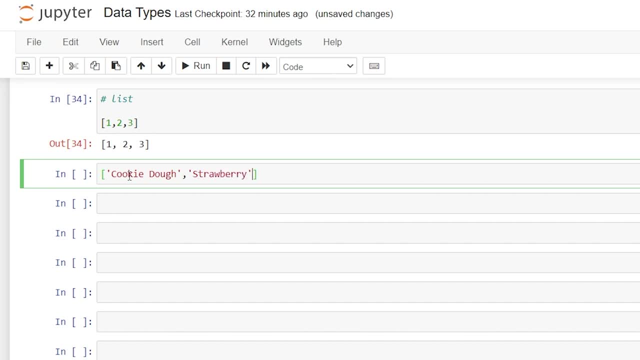 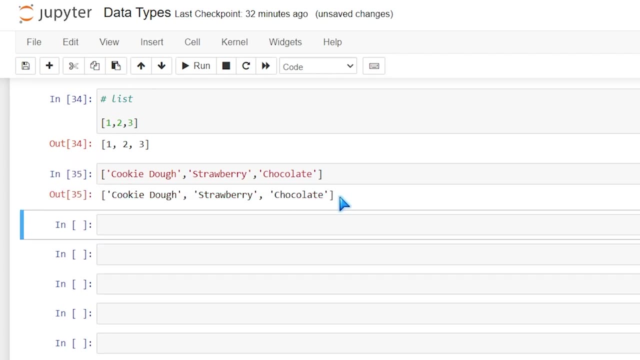 and then we'll say strawberry, and then we'll do one more, and this will just be chocolate, And when we run this, we have all three of these values stored in our list. Now, one of the best things about lists is you can have any data type. 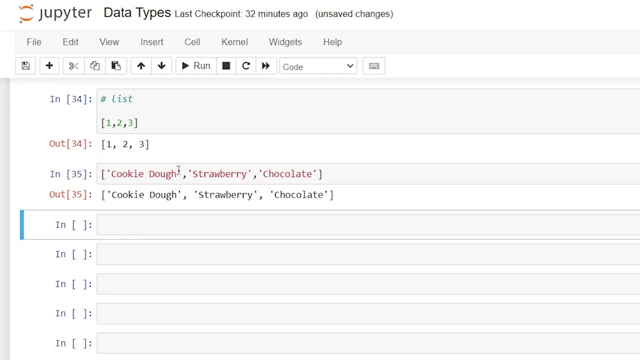 within them. They don't just have to be numbers or strings. You can basically put anything you want in there. So let's create a new list and let's say vanilla, And then we'll do three, and then we'll add a list within a list and we'll say: 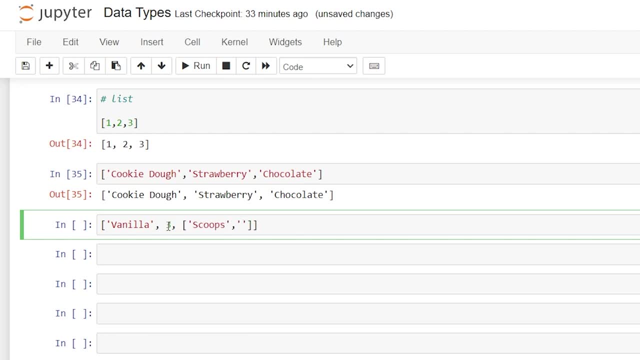 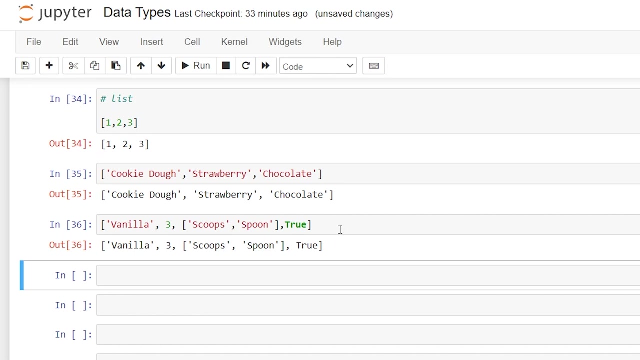 scoops, comma spoon, and then we'll get out of that list and then we'll add another value of true for boolean And now we can hit shift, enter and we just created a list with several different data types within one list. Now let's take this one. 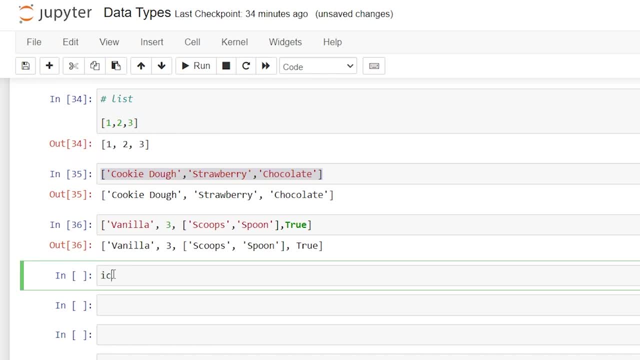 list right here with all of our different ice cream flavors. We'll say ice- I'm going to underscore cream- is equal to this list. Now, one thing that's really great about lists is that they are changeable. That means we can change the data in here. 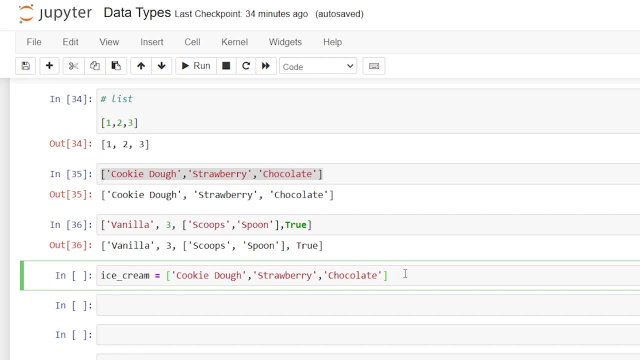 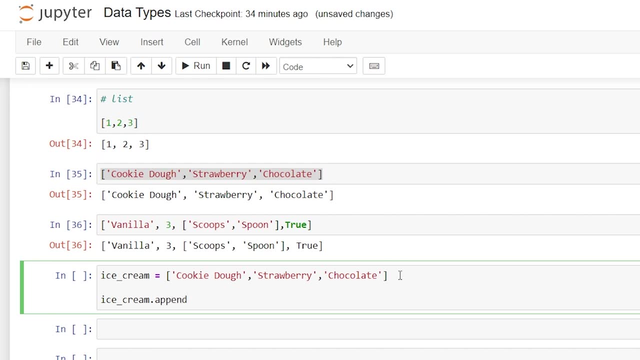 We can also add and remove items from the list after we've already created it. So let's go and take ice cream and we'll say ice cream dot. append- And this is gonna do- append it to the very end of the list. Do an open parentheses and let's say salted caramel. 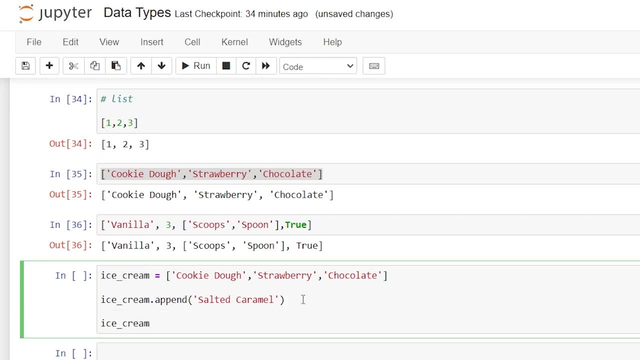 Now, when we run this and we call it, just like this, it's gonna take this list, add salted caramel to the end and we'll print it off. And, as you can see, it was added to the list And, just like I said before, let me go down here. 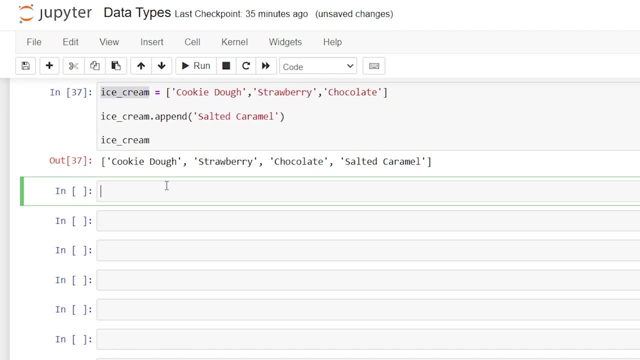 We can also change things from this list. So let's say ice cream, and then we need to look at the indexed position. So we're gonna say zero and that's gonna be this cookie dough. right here We can say that is equal to. so we can now change that value. 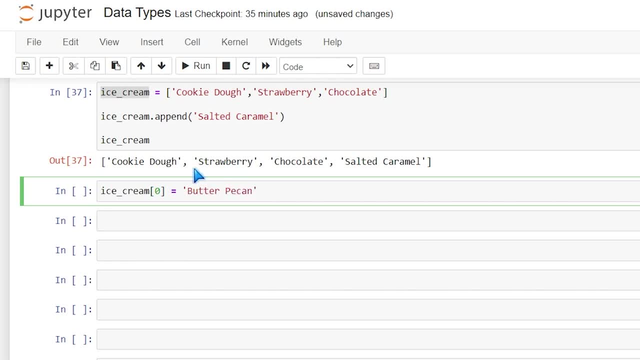 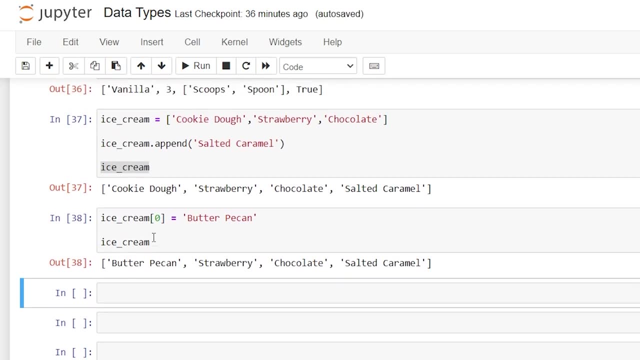 So let's call that butter pecan, And now, when we call it, we can now see that the cookie dough was changed to butter pecan. Another thing that you saw just a little bit ago is something called a list within a list, basically a nested list. 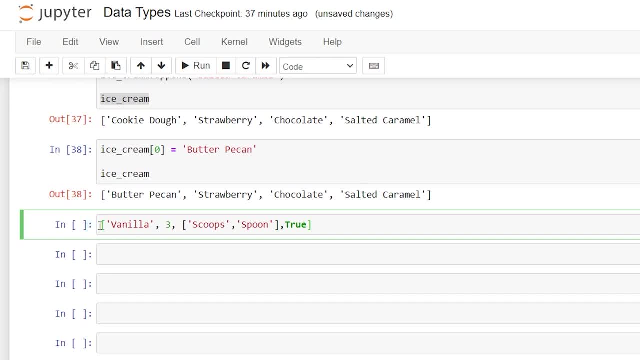 So we had scoops spoon. true, Let's give this and we'll say: nested underscore list is equal to Now. when we run this, we now have this nested list. So if we look at the index, we have the list. 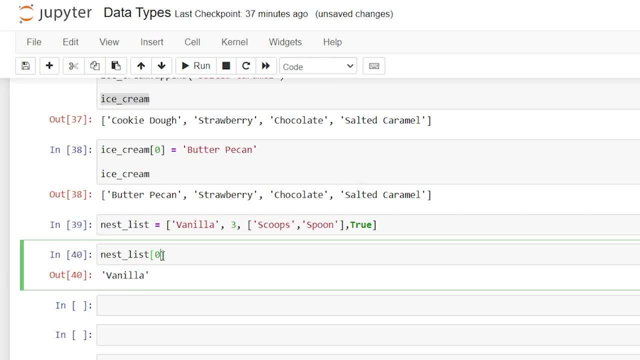 and we say 0,, we'll get vanilla. If we say 2,, we'll get scoops and spoons. Now, since we have a list within a list, we can also look at the index of that nested list. So let's now say 1. 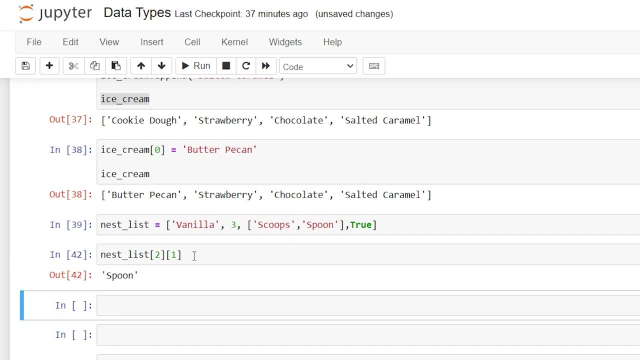 and that should give us just spoon. And you can go on and on and on with this. You can do lists within lists within lists, and all of them will have indexing that you can call. Now let's go down here and start taking a look at tuples. So a list and a tuple are actually quite similar. 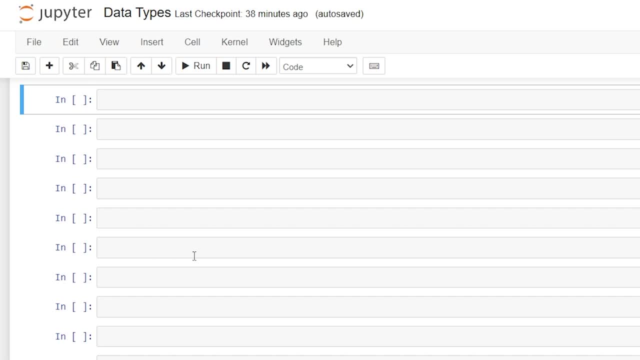 but the biggest difference between a list and a tuple is that a tuple is something called immutable. It means it cannot be modified or changed after it's created. Let's go right up here. We're going to say tuple and let's write our very first tuple, So we'll say tuple underscore. 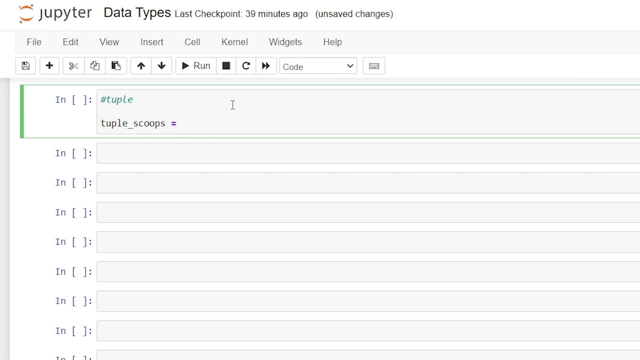 scoops is equal to, and then we'll do an open parentheses. Now, these open parentheses, you've seen, if you do like a print statement, but that's different because that's executing a function. This is actually creating a function. So we're going to do a print statement, So we're going to 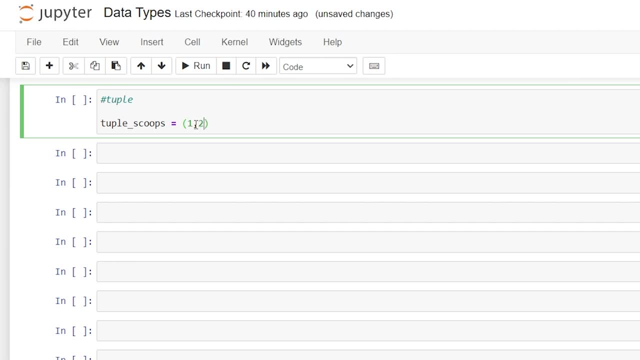 create a tuple which is going to store data for us. So we'll say 1, 2, 3, 2 and 1.. Let's go ahead and create that tuple and we can just check the data type really quickly. And it's a tuple And just. 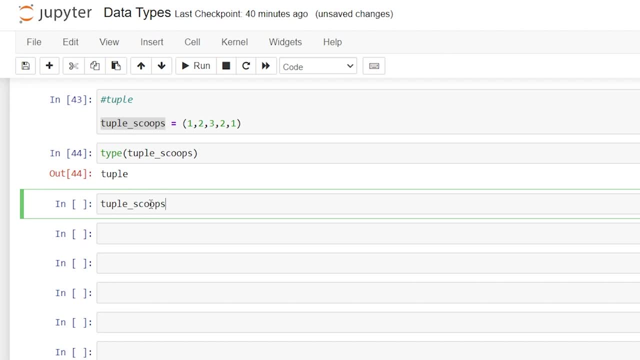 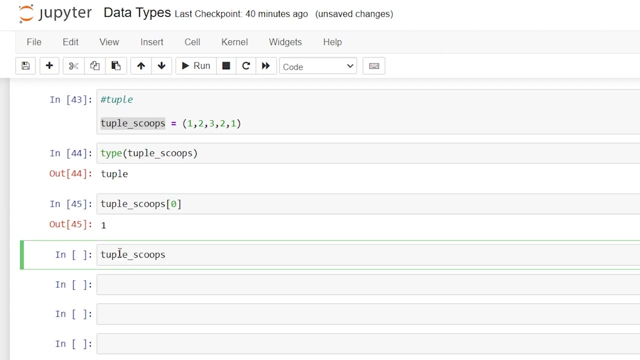 like we saw before, a tuple is also indexed. So if we go at the very first position, which is a 1, we will get the output of a 1.. But we can't do something like append and then add a value like 3.. If we do that, we're going to get a 1.. And if we do that, we're going to get a 1.. And if we do that, 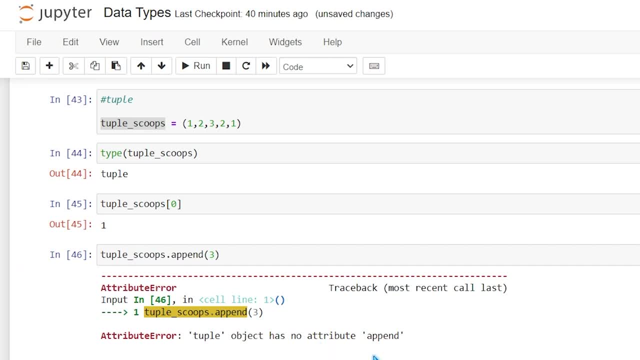 it's going to say: tuple object has no attribute append. It's just because you cannot change or add anything to a tuple, just like we were talking about before. Typically, people will use tuples for when data is never going to change. An example for this might be something like a city name. 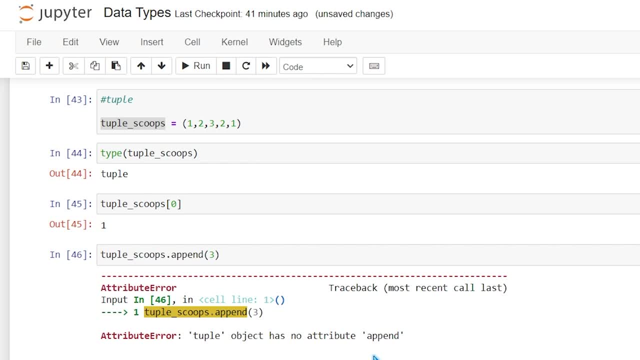 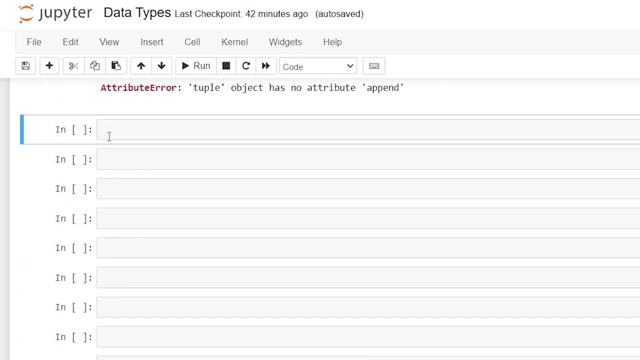 a country, a location, something that won't change. They definitely have their use cases, but I don't think they're as popular as just using a list. So now let's scroll down and start taking a look at sets. But really quickly, let me add a few more cells. 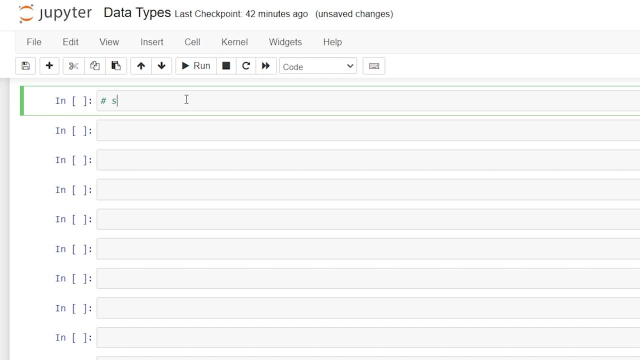 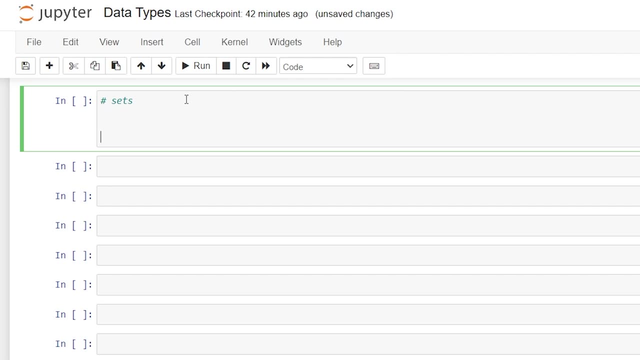 And let's say sets. Now, a set is somewhat similar to a list and a tuple, but they are a little bit different in the fact that they don't have any duplicate elements. Another big difference is that the values within a set cannot be accessed using an index because it doesn't have an index. 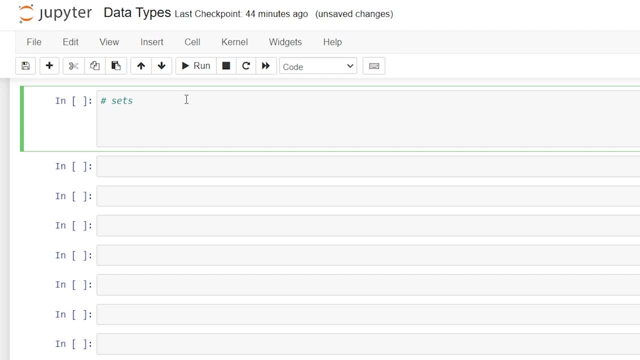 because it's actually unordered. We can still loop through the items in a set with something like a for loop, but we can't access it using the bracket and then accessing its index point. So let's go ahead and create our very first set. So we're going to say daily underscore pints. 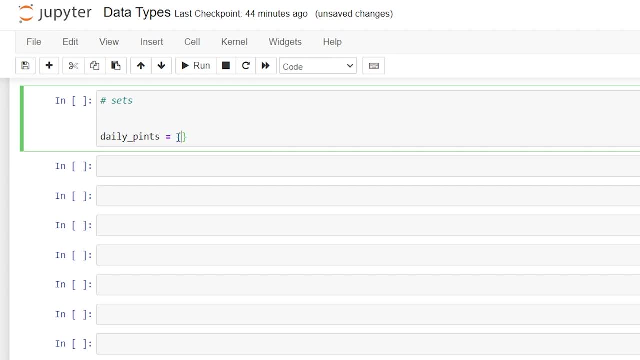 Then we're going to say equal to and to create a set. we're going to use these squiggly brackets- I don't know if there's an actual name for those. if I'm being honest, I call them squiggly brackets and that's what we're going to go with. We're going to put in a one, a two and a three. 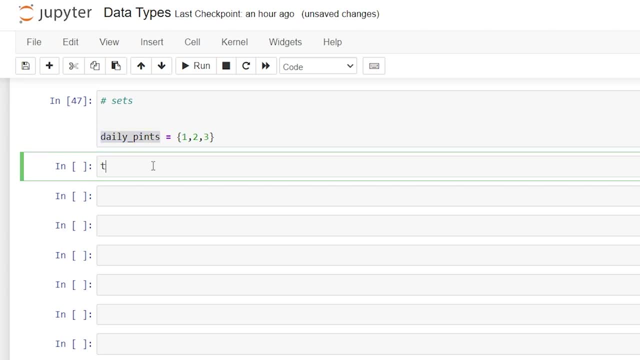 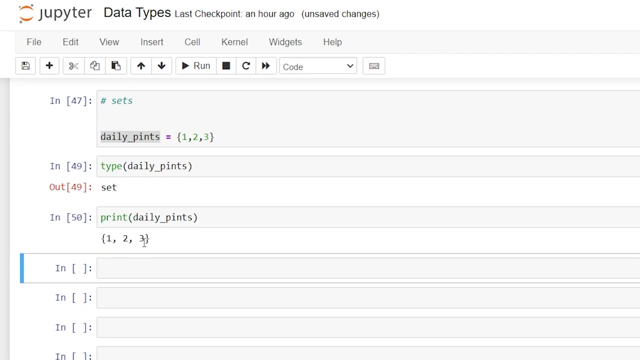 So let's go ahead and run this and let's look at the type And, as you can see, it is a set. Now, when we print this out, it's going to show us one, a two and a three and those are all the values within our set. But if we copy this and we'll say daily, 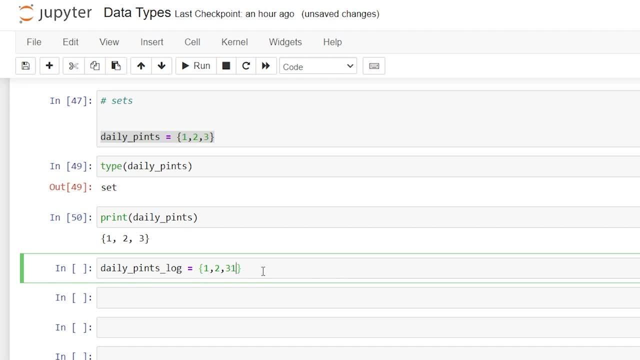 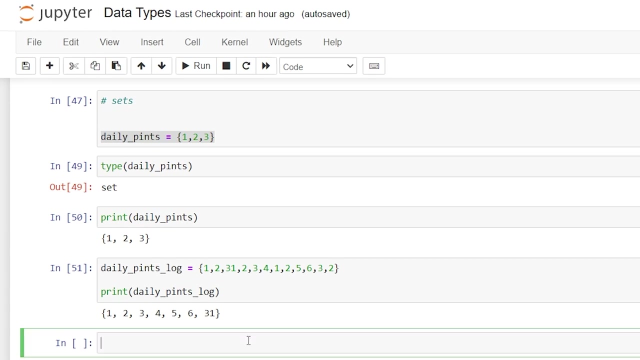 pints log. this is going to be every single day. Maybe I had different values. Now, when we run this and we do the exact same thing, Now when we print this, it's going to have just the unique values within that set. Now a use case for set, and this is something that I've done in the past. 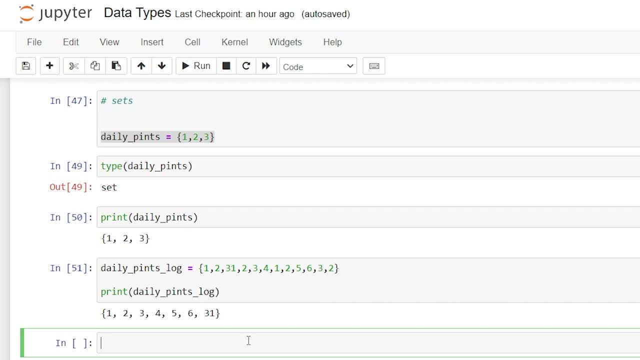 is comparing two separate sets. Maybe you have a list or a tuple and you convert that into a set and that will narrow it down to its unique values. Then you can compare the unique values of one set to the unique values in another set and then we can see what's the same and what's. 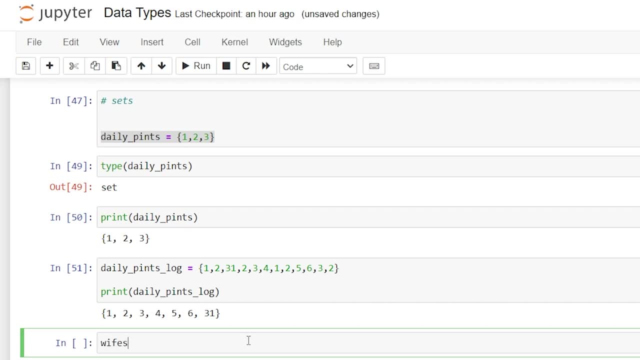 different. So let's go down here and let's say wife's underscore daily, and we'll just copy this right here. We'll say is equal to: let's do our squiggly lines, Let's do one, two, Let's do just random numbers. So now, this is my daily log and this is my 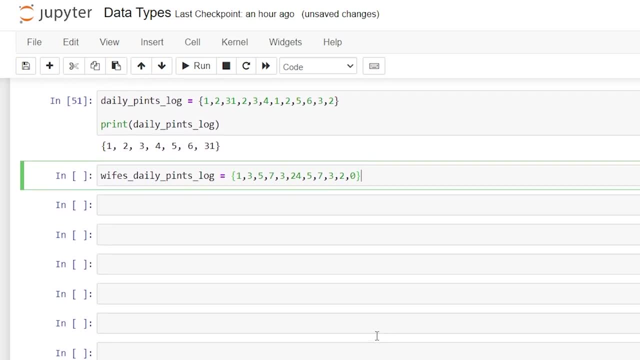 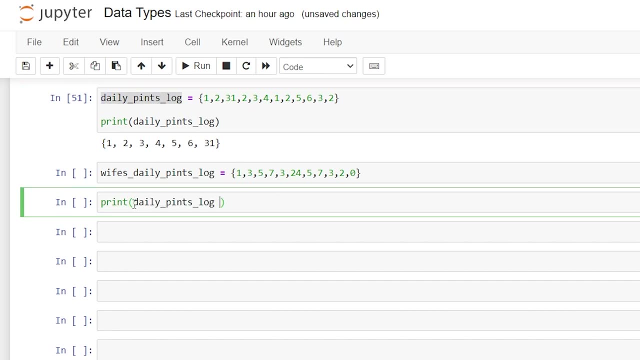 wife's daily log And now we can compare these values. So let's go right down here, Let's say: print We'll do my daily logs and then we'll do this bar right here And this is going to show us the combined unique values. It's basically like putting them all in one set and then trimming. 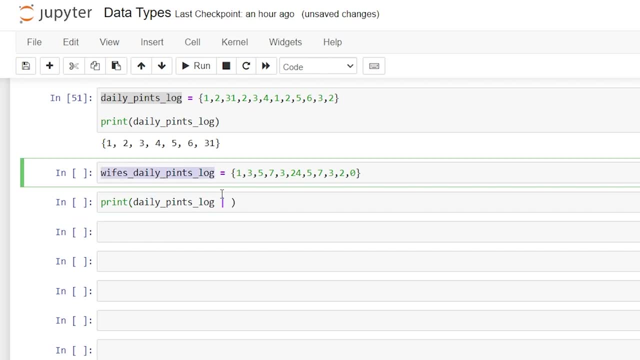 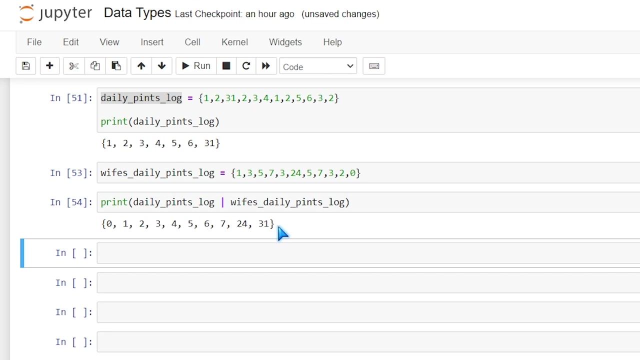 it down to just the unique values. So we'll take wife's daily pints log And when we run this, we actually need to run this first. When we run this, we should see all the unique values between these sets And so, as you can see, 0, 1, 2, 3, 4, 5, 6, 7, 24, 31.. So these are all the unique values between these. 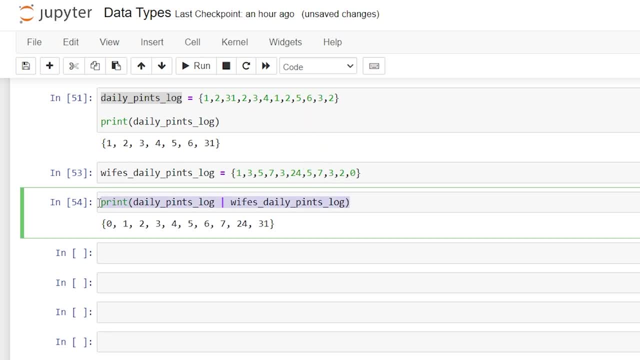 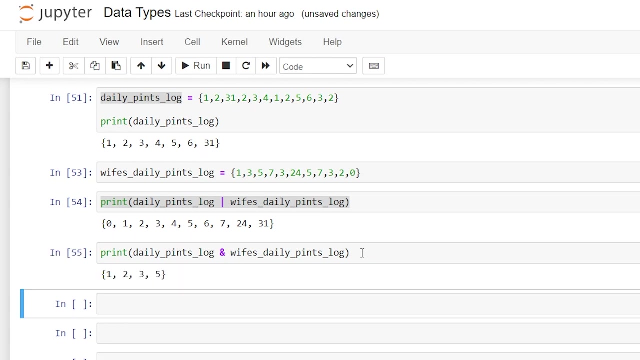 two sets, We can also do another one, And instead of this bar we're going to do this symbol right here, which I believe is called an ampersand. Don't quote me on that, But when we run this it's going to show what matches- That means which ones- show up in both sets, So the only ones that show up in. 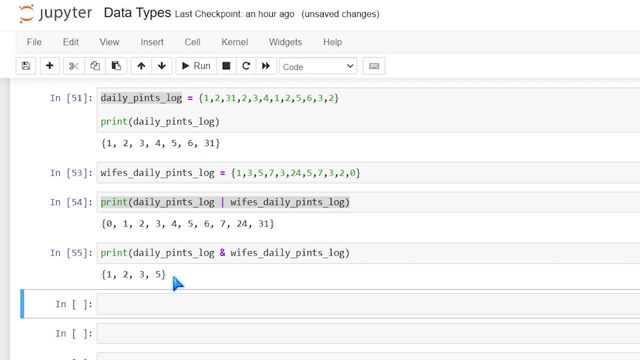 both sets are 1, 2, 3 and 5. We can also do the same thing here. We can also do the same thing here. We can do the same thing here. We can also do the same thing here. We can also do the same thing here, We can. 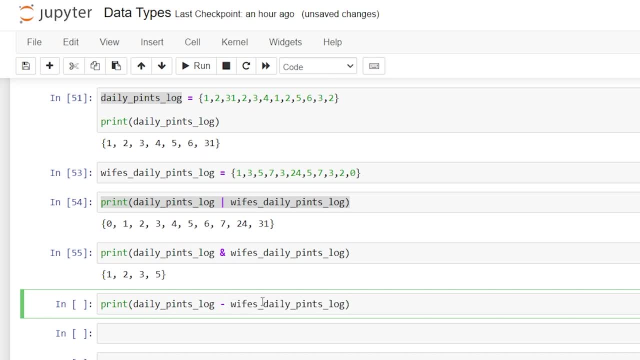 also do the opposite of that by doing a minus sign, And this is going to show us what doesn't match. So we have 4, 6 and 31.. Now where is our 24? that was in our wife's daily pints log. It's in. 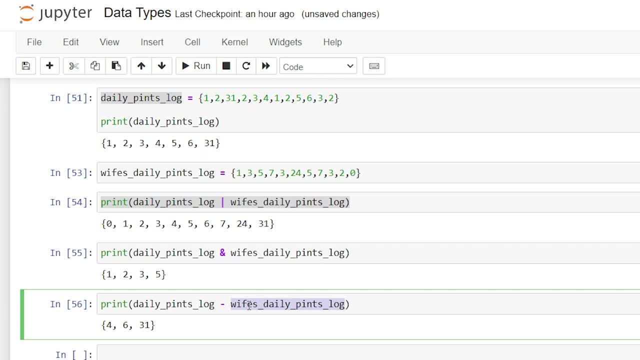 this one, but we're subtracting the values on this one. So let's reverse this and we'll say: daily pints, log And let's run it Now. those are our other values. So we're taking the values of this and then we're subtracting all the ones that are the same and getting the remaining values. 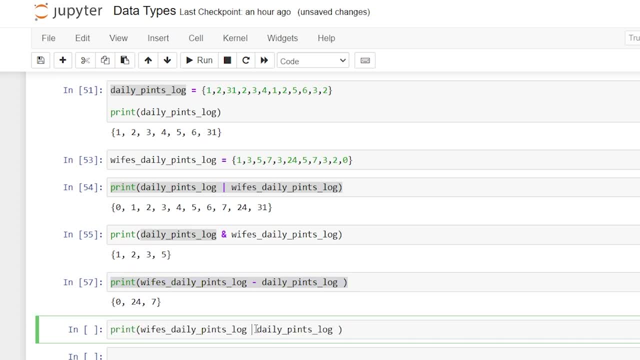 And then for our last one, we can get rid of this and we'll do this symbol right here, And this is going to show if a value is either in one or the other, but not in both. So let's run this. So these values are completely unique only to each of those sets. Now, the very last one that we are going to. 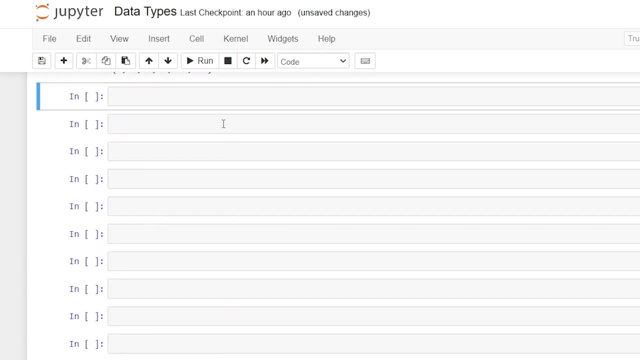 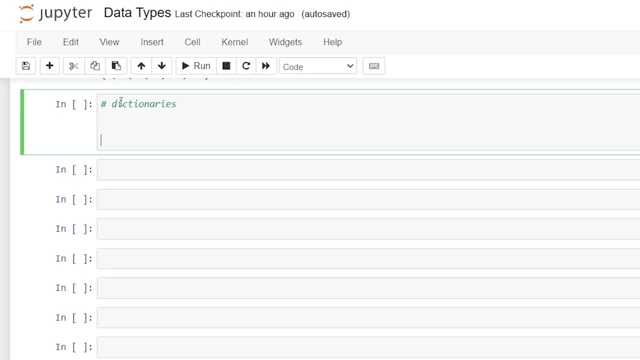 look at in this video is dictionaries. So let's go right down here, Let's add a few cells and let's say dictionaries. Now I saved dictionary for last because this one is probably the most different out of all the previous data types that we've looked at. Within a data type, we have something called a key value. 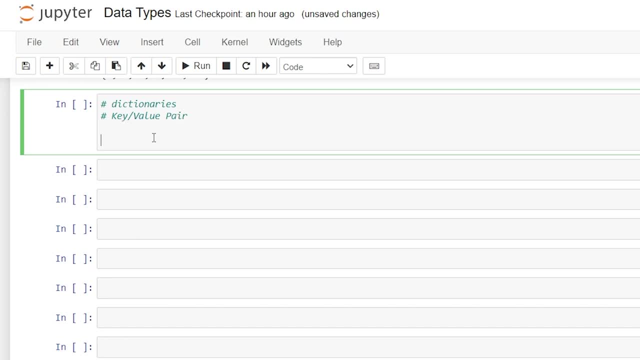 pair. That means when we use a dictionary. it's not like a list where you just have a value, comma value, comma value. We have a key that indicates what that value is attributed to. So let's write out a dictionary to see how this looks. We're going to say dictionary, underscore cream and. 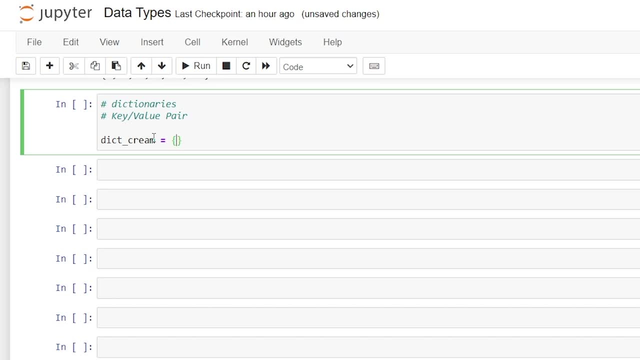 just like a set. we use a squiggly line, But the thing that differentiates it is that in a dictionary we'll have that key value pair, whereas in a set each value is just separated by a comma. So let's write name and this is our key, and then we do a colon, and this is then where we input our value. 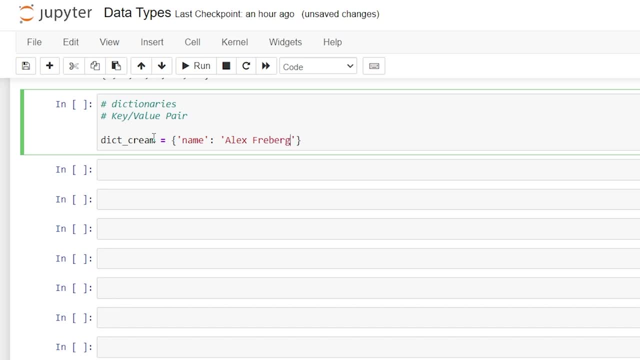 So we're going to say Alex Freberg, and then we separate that key value pair by a comma. and now we can do another key value pair. So we'll say weekly Intake and a colon, and we'll say five pints of ice cream, the comma, and then we'll do favorite ice. 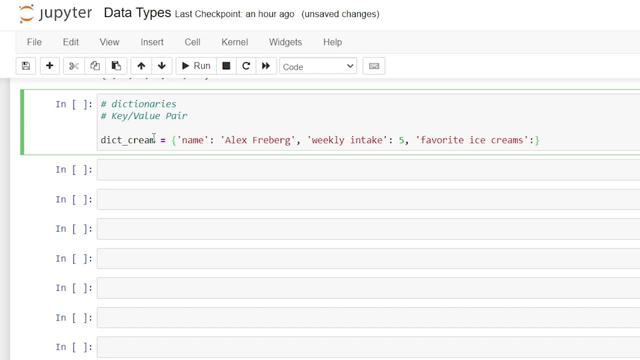 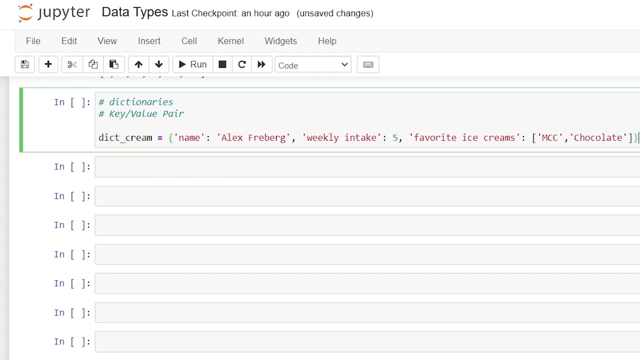 creams. And now what we're going to do is we're going to put in here a list, So within this dictionary we can also add a list. We'll do MCC for mint chocolate chip and then we'll add chocolate- Another one of my favorites. So now we have our very first dictionary. Let's copy this and run it. 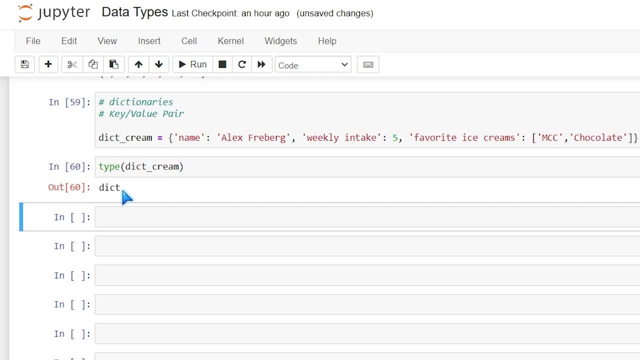 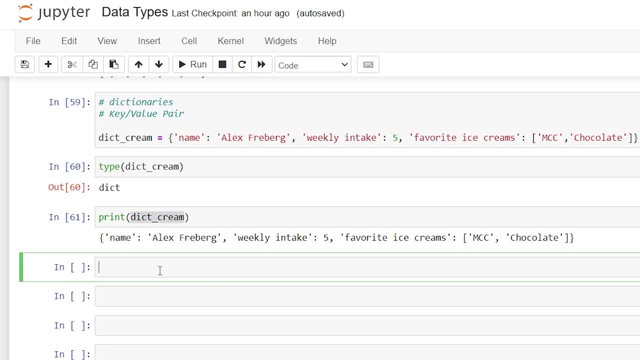 and let's just look at the top Type And, as you can see, it says that this is a dictionary. Let's also print it out Now. if we want to, we can take our dictionary cream and say dot values with an open parentheses When we execute. 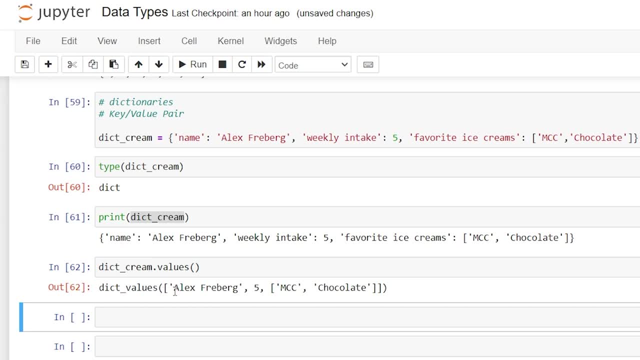 this. we'll see all of the values within this dictionary. So here's our values of Alex Freberg, five, mint, chocolate chip and chocolate. We can also say keys And when we run this, all of the keys: the name, weekly intake and favorite ice creams. 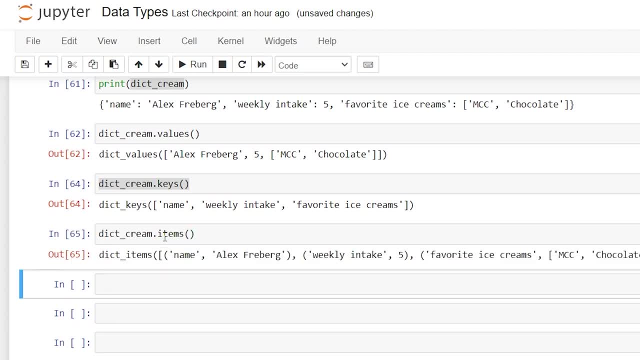 And We can also say items. So this key value pair is one item and this key value pair is another item. Now, one difference between something like a list and a dictionary is how you call the index. But you can't call it by doing something like this where you just do a bracket, oops, and say zero. 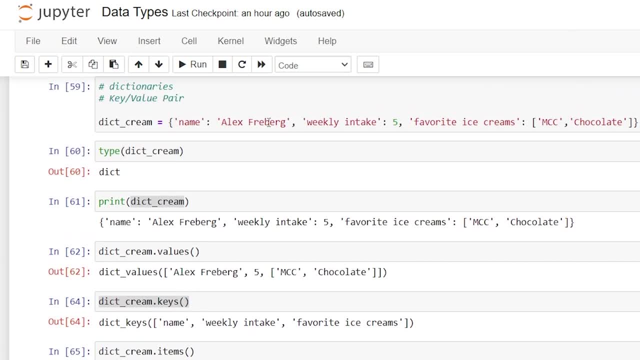 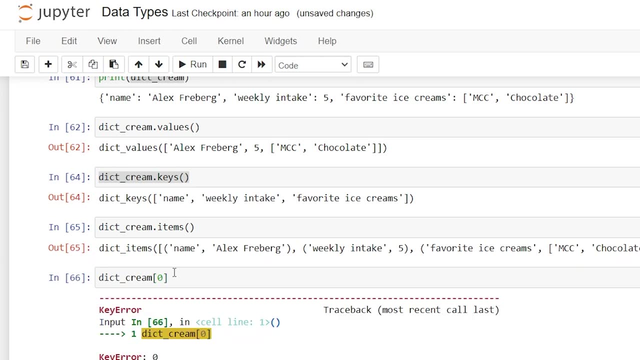 So this would, in theory, take this very first one right, Our very first key value pair. That's going to give us an error. How you call a dictionary is actually by the key, So it doesn't technically have an index, but you can specify what you want to call and take it. 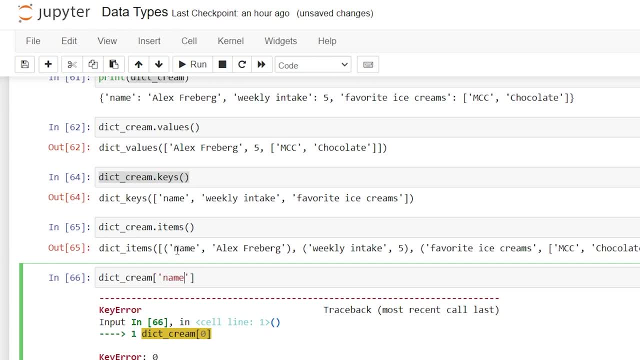 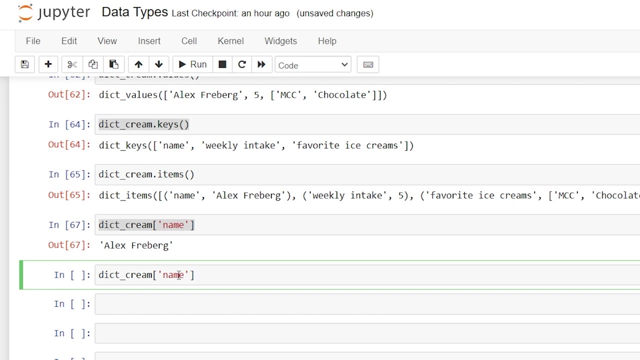 out. So we're going to say name and this is going to call that key right here, And when we run this, we'll get the value, which is Alex Freberg. One other thing that you can do is you can also update information in a dictionary, which we can't with some other data types. So for this, for the name, it. 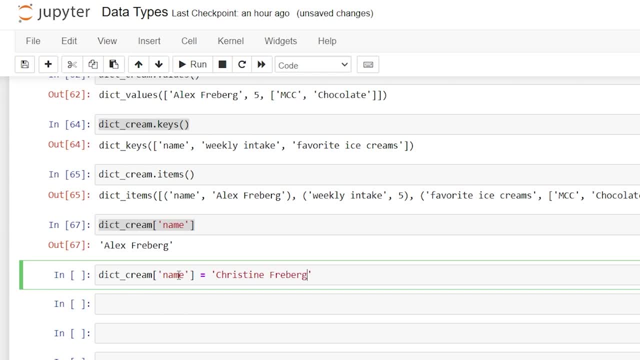 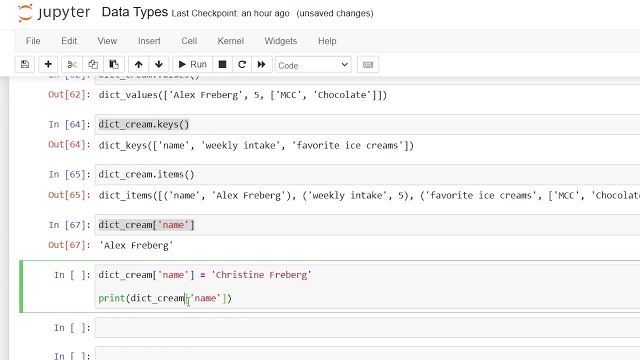 was Alex Freberg. Now let's say Steen Freberg, And when we update that, I'm also going to print The dictionary. it was this. So it's going to update Christine Freberg in that value of the name. So let's go ahead and run this. and now it changed the name. 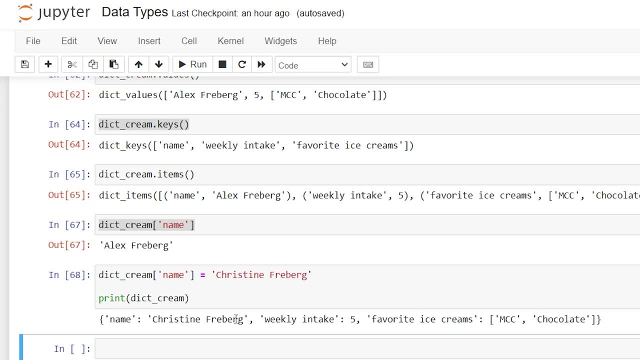 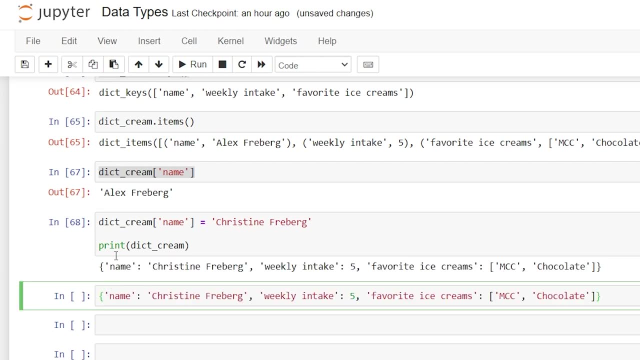 from Alex Freberg to Christine Freberg. We can also update all of these values at one time. So let's copy this And I'm gonna put it right down here. I'm gonna say dictionary- dot, cream, dot, update. Then we're gonna put: 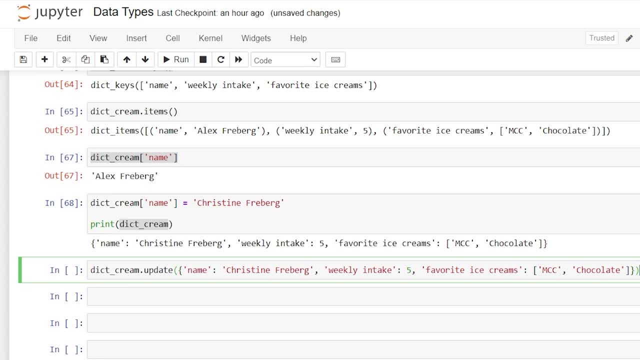 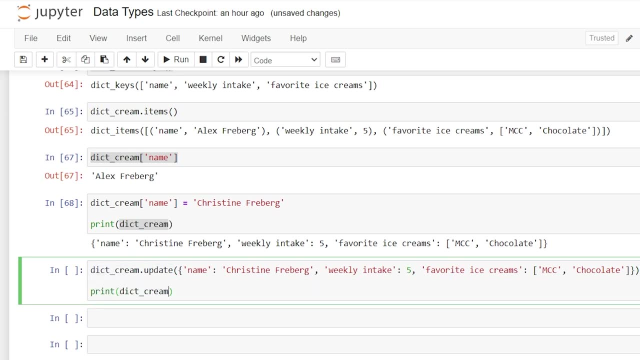 a bracket or not a bracket, but a parentheses around these. so now what we're gonna do is update this entire thing. let me take this, say: print this dictionary. now we can update this to anything we want. so instead of here I can say I'll say wait, and because of all that ice cream, I now weigh 300 pounds. so 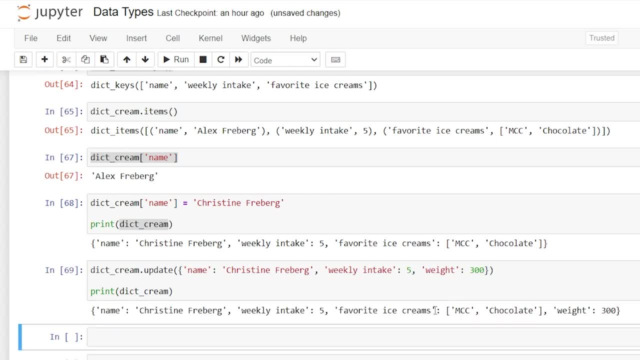 let's run this and, as you can see, it did not delete our key value pair right here. instead, it just added to it. when you're using the update, we can't actually delete. that's the delete statement and I'll show you that in just a second. but all we did was added this new value. it also is going to check and